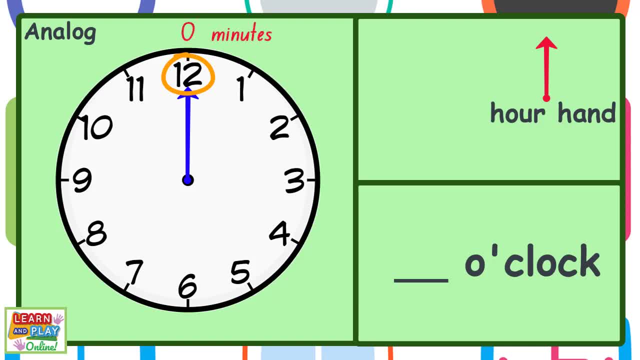 number 12, that means that no minutes have passed the hour. We also already know that the number that the hour hand is pointing to will tell us what hour we are in. So what is the time? on the clock, It is two o'clock. 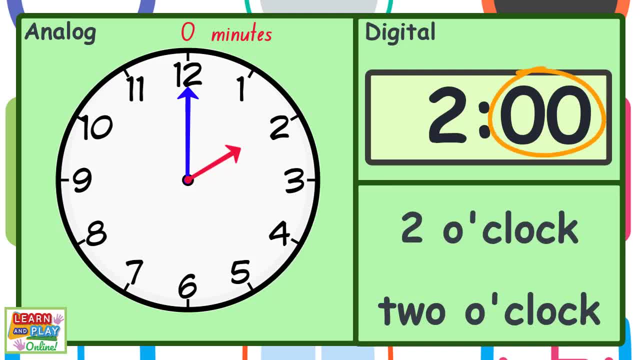 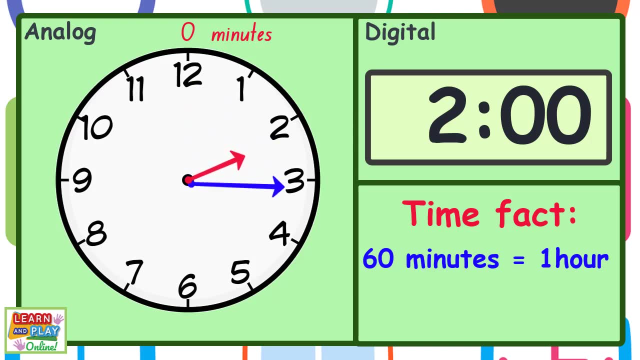 Take notice that the minutes section on the digital clock says zero. This means that zero minutes have passed the hour. Here is a time fact: There are 60 minutes in one hour. So that means when the minute hand does a full rotation around the clock face, 60 minutes has passed and it will take us. 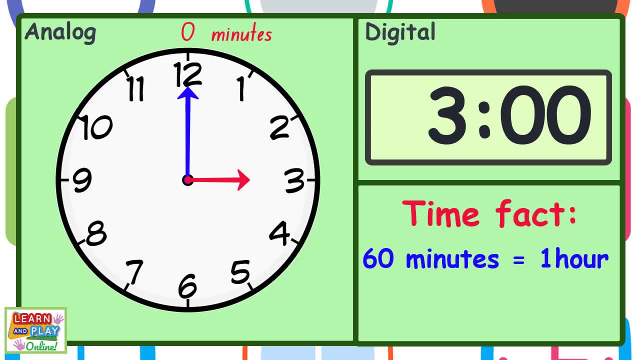 into the new hour. In this case, it is now three o'clock. Now let's see what happens when the minute hand travels halfway around the clock. Since the minute hand has traveled only halfway around the clock, it is now pointing at the number. 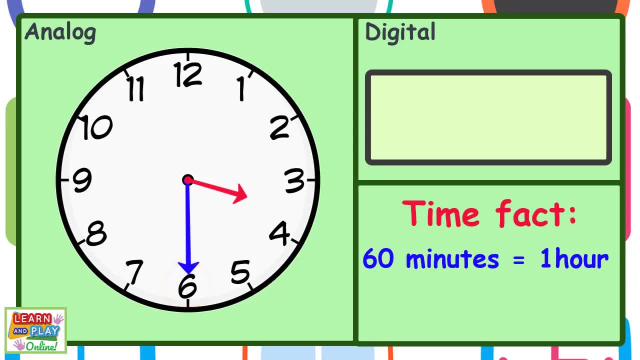 six. Now we already know that one full rotation of the minute hand is equal to 60 minutes. If we count this by CARV 2, we see that as 30. So that means that half a rotation is equal to 30 minutes, Because half of 60 minutes is 30 minutes. 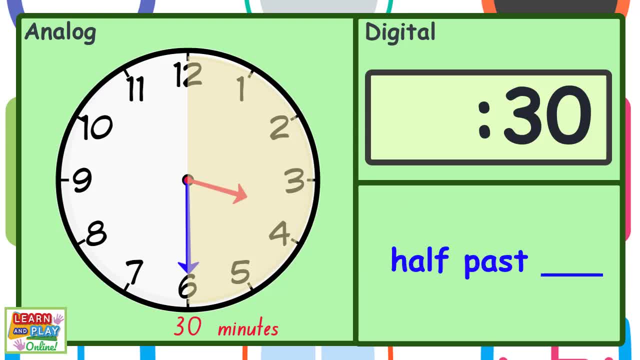 That's also why when the minute hand is pointing to the 6, we say it is half past something, because the minute hand only went halfway around the clock. That is also why on the digital clock in says 30, indicates 30 minutes has passed the hour. now let's have a look at where the hour hand is pointing. 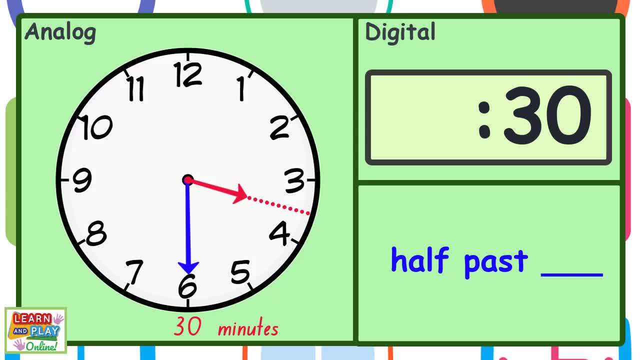 as you can see, the hour hand is right in between the numbers three and four. this means that it has passed three and has not yet reached the number four. that is why we say it is half past three, or 3: 30.. let's watch the minute hand. do a full rotation from where it is now. 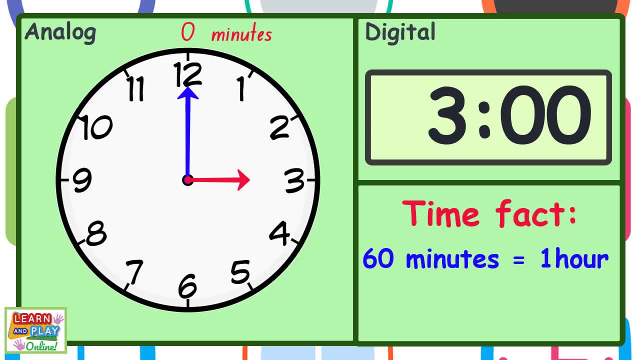 into the new hour. In this case, it is now three o'clock. Now let's see what happens when the minute hand travels halfway around the clock. Since the minute hand has traveled only halfway around the clock, it is now pointing at the number. 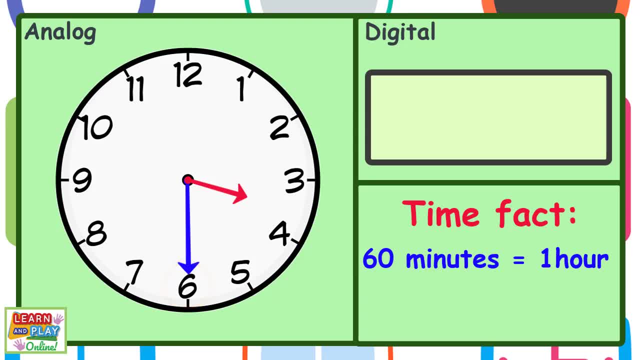 six. Now we already know that one full rotation of the minute hand is equal to 60 minutes. Take a look at the number six in the digital clock. The minute hand is now pointing at the number six, So that means that one part of the rotation 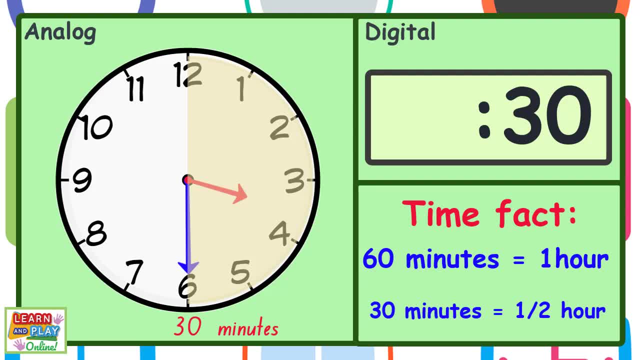 is equal to 30 minutes, because half of 60 minutes is 30 minutes. That's also why, when the minute hand is pointing to the six, we say it is half past something, because the minute hand only went halfway around the clock. on the digital clock it says 30 because it indicates 30 minutes has passed the 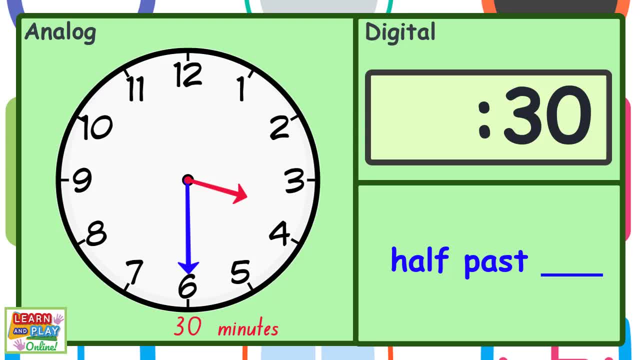 hour. now let's have a look at where the hour hand is pointing. as you can see, the hour hand is right in between the numbers 3 & 4. this means that it has passed 3 and has not yet reached the number 4. that is why we say it is half. 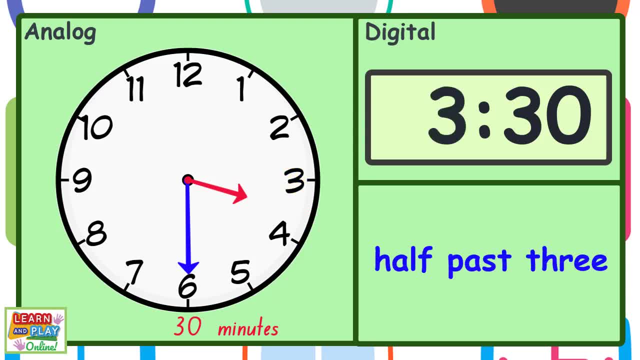 past 3 or 3, 30. let's watch the minute hand to a full rotation from where it is now, so we can see that the minute hand is pointing to the number 6, which means it is half past something. the hour hand is in between the numbers 4 & 5, which 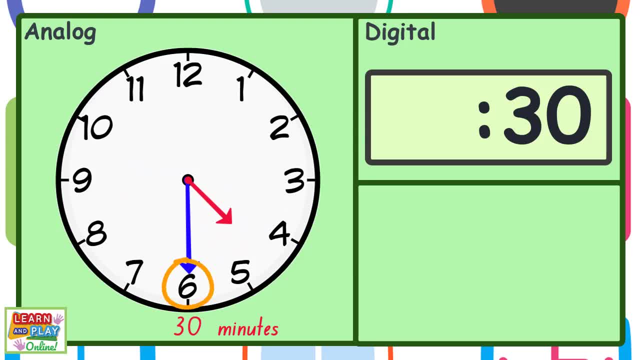 so we can see that the minute hand is pointing to the number six, which means it is half past something. the hour hand is in between the numbers four and five, which means that it has gone past the four and has not yet reached the number five. so we can see that the hour hand is pointing to. 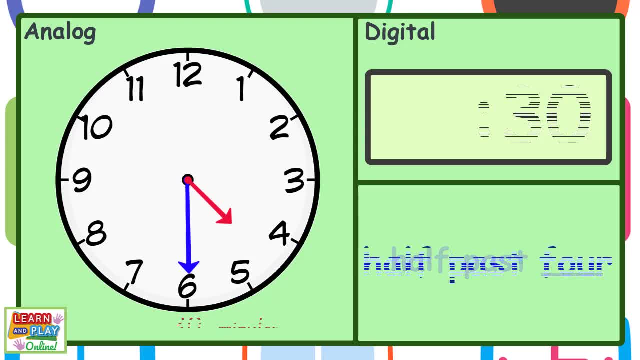 not yet reached the number five, so the time is half past four or 4, 30.. now that you have learned how to read half past times, let's practice reading the times on the clock coming up half past 10 or 10, 13.. 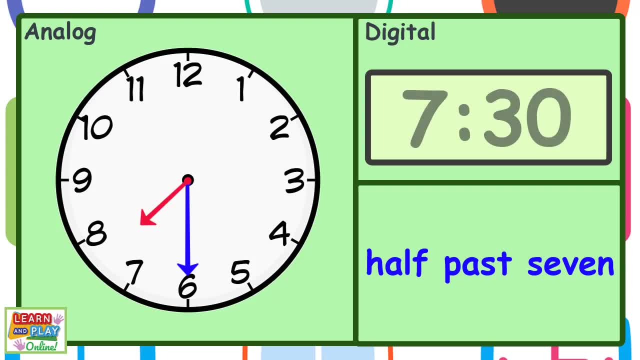 half past seven or half past seven or 7: 30.. half past one or 1: 30.. half past eight or 8: 30.. half past 11 or 11: 30.. half past 11 or 11: 30.. 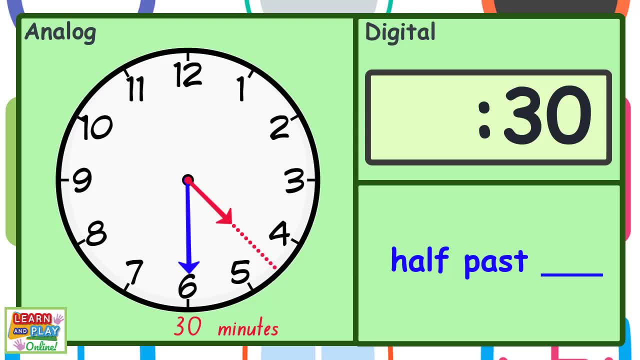 means has gone past the four and has not yet reached the number five. so the time is half past four or 4, 30.. now that you have learned how to read half past times, let's practice reading the times on the clock coming up: half past 10 or 10, 30. half past 7 or 7, 30. 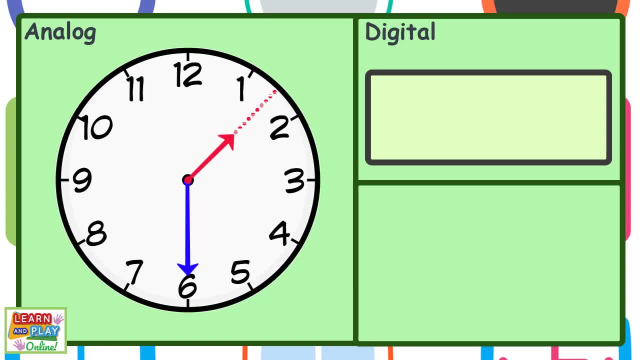 half past: 1 or 1, 30 half past, 8 or 8, 30 half past. 11 or 11, 30 half past. 11 or 11, 30 half past. 2 or 2, 30 half past, 2, 5, 30. 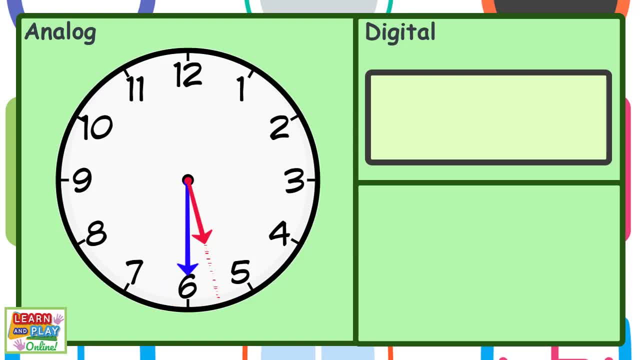 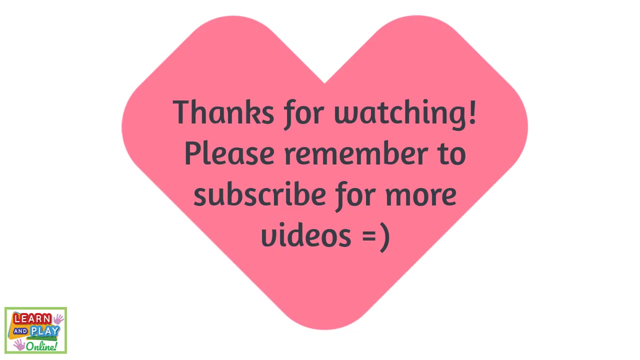 half past 4, 5, 30, half past 5 or 5, 30, half past 3 or 4, 30, Half past twelve or twelve-thirty, Half past nine or nine-thirty, Half past six or six-thirty. Thanks for watching. Please remember to subscribe for more videos.